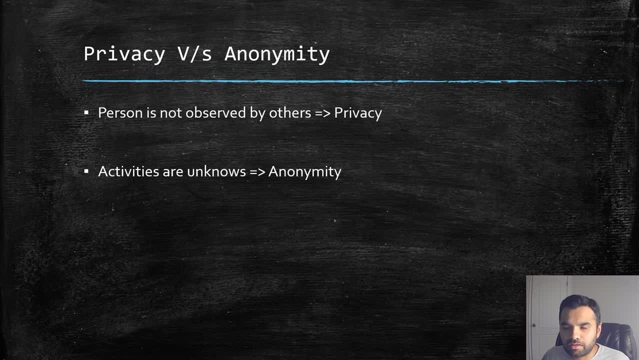 mask or kind of a mask, and washing your car in the garage, People would know that, oh, somebody is washing the car, but they don't know who is washing the car. That's an anonymity. So that's a basic difference between what's the privacy and what's anonymity. This is very 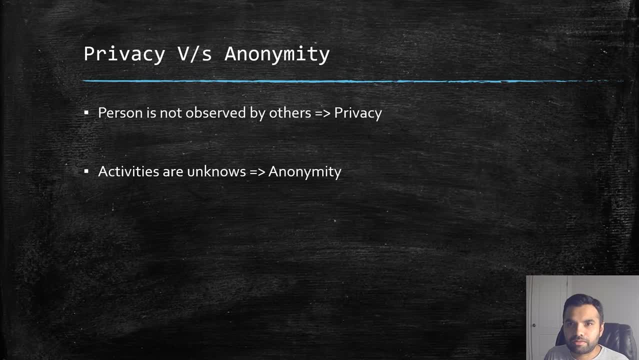 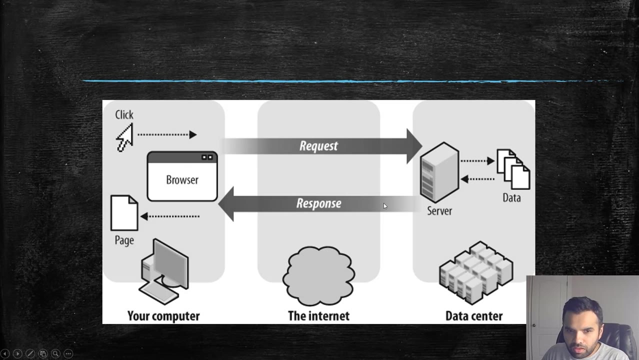 very critical When you access, and When you access and you think about, like you know, the dark web services, uh, how do you maintain both of this, uh, to be able to uh keep yourself anonymous and and still be able to access all the services, okay, so, since we have this clear, uh, the next question comes: why does the normal activity that 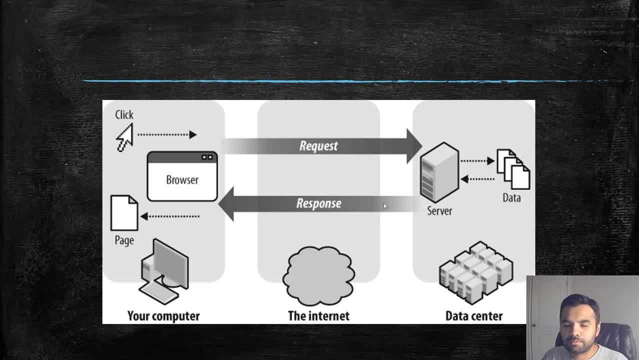 we perform uh through our, through our local, local system, uh, we cannot have privacy or anonymity. uh. the reason for that is suppose you have uh, like you know, you're using some some basic browser like chrome or firefox, and you're sending a request uh to the server, let's say, googlecom. which is of course first going to go to the ips, your internet service provider, and then it will go to the maybe different nodes and then finally hit to the googlecom and then it will come back to the. it will send the response back now at various points. uh, especially when the traffic. 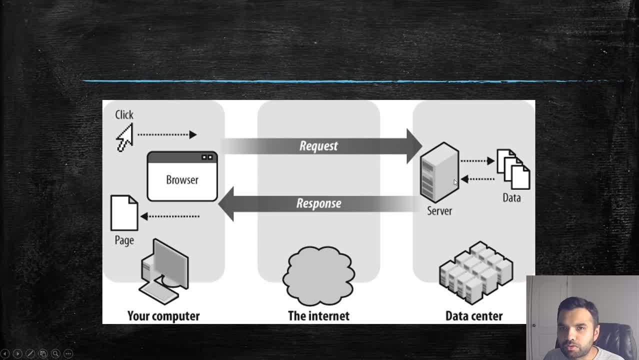 leaves your browser and goes to the server. it will send the response back to the server and then it will come back to the. it will send the response back now at various points, especially when the, the isp, and then it goes to the server. it's a various uh. there are various data points where 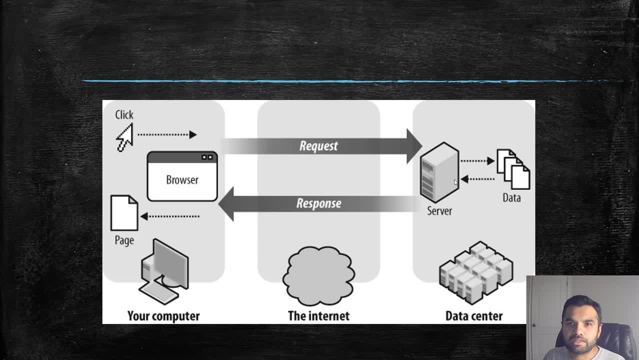 your isp could sniff what you are doing. uh, there is a government agency who can sniff what activity you are doing and who is doing. it has all the details about, like you know, where the traffic is coming from, your ip address and, and all the information and same thing. uh, like in the google. 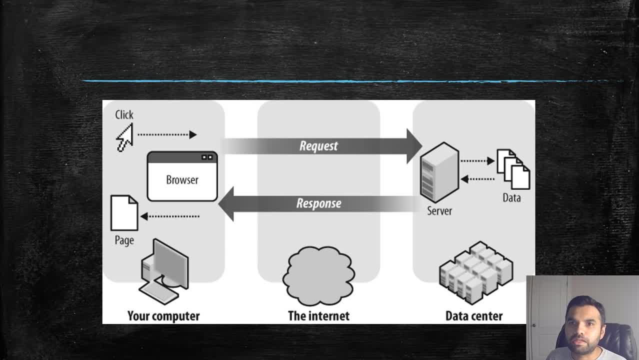 as well, like if you are, let's say, going to googlecom, it can also have, it can also find all the details uh about. you know who is making the requests and where the request going. so there is no privacy uh or anonymous aspect, and- and now nowadays you must have seen a lot of uh pop-ups in. 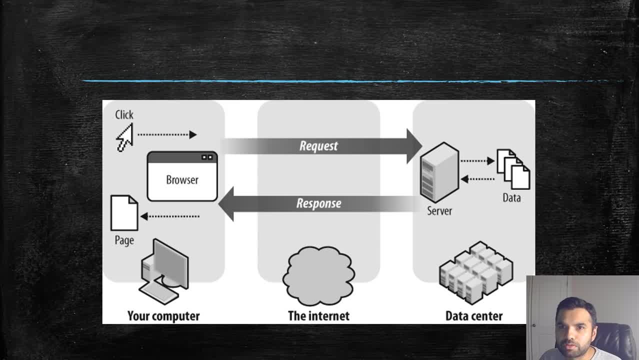 in various websites that you're visiting. that it's they're using the cookies for the privacy- uh, not the privacy, but actually collecting the data. uh, whether you you're okay with that or not. so those are the. those are the reasons. uh, dark web services. you cannot access with this normal browsers, because 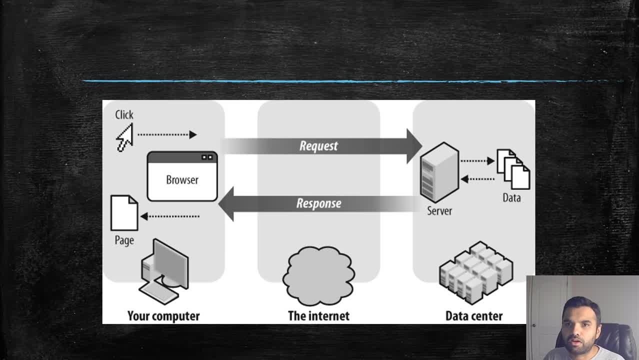 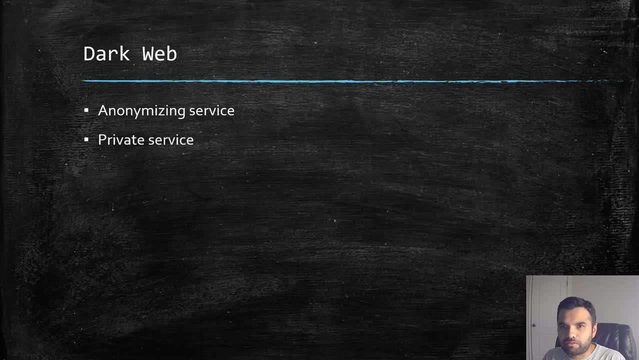 of course, uh, you are not anonymous, your identity will not be, uh will not stay anonymous or private. so, to access the dark web or what we? what? what do we mean by the dark web? so the dark web services, uh, are made up of two, two aspects. one, we need the anonymizing service. so, uh, the service which would 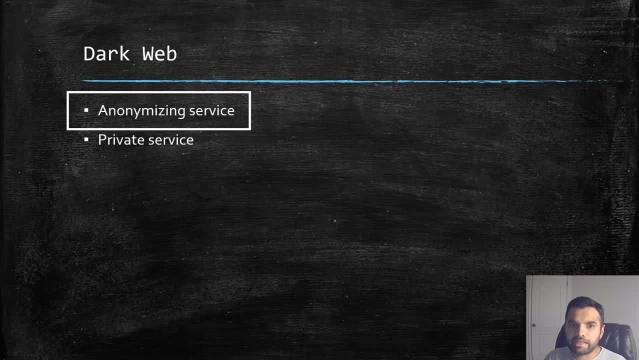 keep everything anonymous, uh, whatever we do. and then we have to use the private services. now, there are not many services out there. uh, who can, who can, make sure that our, our activity remains the private, or our activity remains the anonymous, and- and that's why there are very selected, uh, number of services. 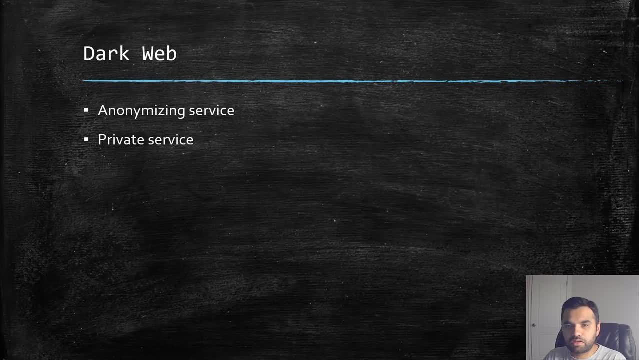 which we're gonna use throughout this, this uh course, or, like you know, next few videos uh, which i'll show you. uh, how do you access the dark web services and and and the and. the third most important thing, which probably i haven't noted here, is the security as well. uh, you have your. 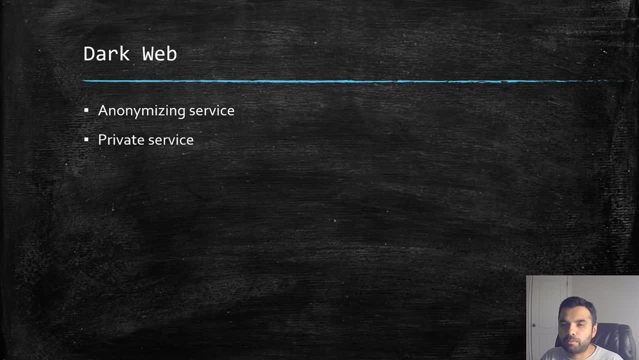 differs, so um you can access it. in this way. you can access your data over here, but you can also access also some of uh the executive accesses which you are using, for example, data analytics. you can access uh your data and uh you know where you have the data, which are all in here. 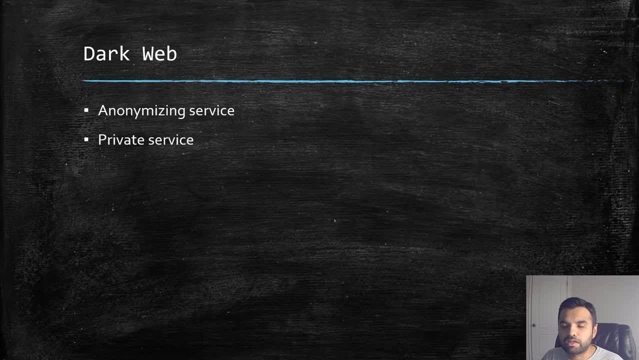 so you can access it. uh, utilizing the dark web services. you can access data analytics too, but you can also access this: uh all the uh, uh, all the uh the uh all the other, uh everything. but if you do not know how to keep it secure, uh other than that, uh just make sure you're using these private services now. so the first, of course. 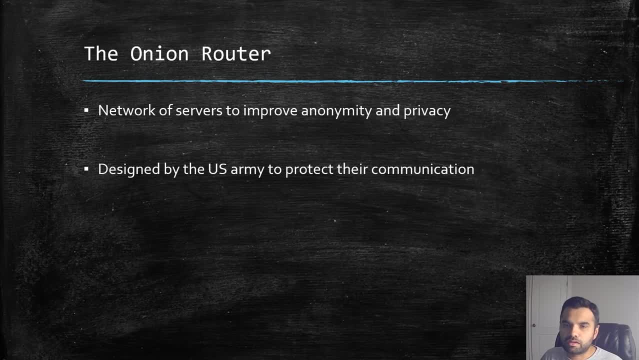 whenever we we call about, like you know, private and being anonymous, the the, like you know, the main thing which comes to the mind is that onion router. it's called tor. so the tor is is the bunch of network servers to improve the anonymity and privacy right and i'm sure you have used, like tor. 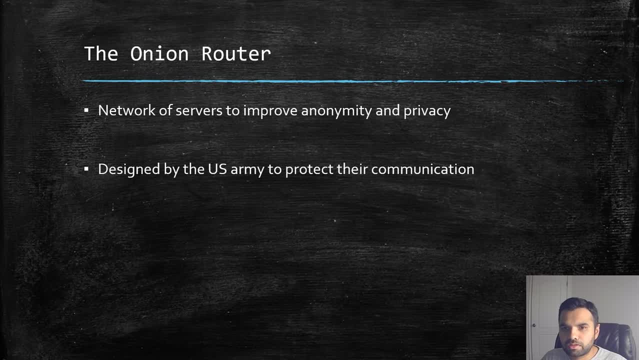 at various point in your career. uh, so tor, tor browser itself might not be uh new to you, but maybe i'll just give you a little bit of brief about how the tor works and then in the following episodes we'll talk more about how to use that. so yeah, the tor essentially is the network of 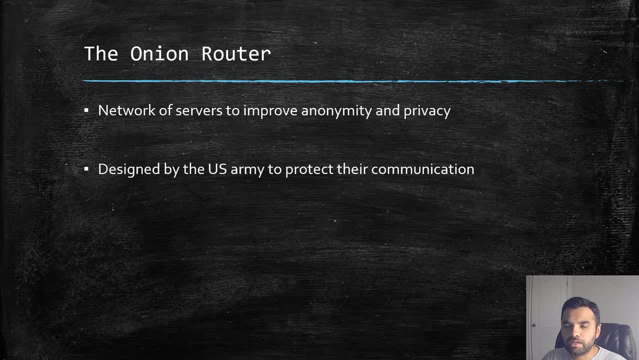 servers to improve the anonymity. so it's a bunch of servers uh made uh to keep yourself anonymous and it's actually designed by the us army to keep their communication secure. uh, like you know, of course, uh for the uh for the different purpose. but yeah, of course uh, that's, that's why the tor was evolved, uh, so why? 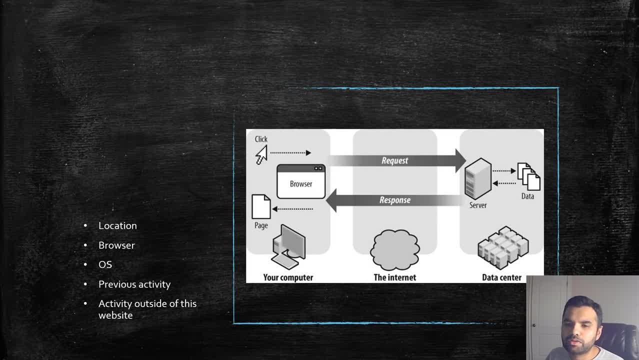 why tor is secure, uh, or why do we need to use tor again? uh, we, we saw this image earlier in the in the video, uh, but, but here, the here is the concern, right? so when you are accessing- uh your any any site, googlecom, from your browser, uh server can obviously locate where the your location browser. 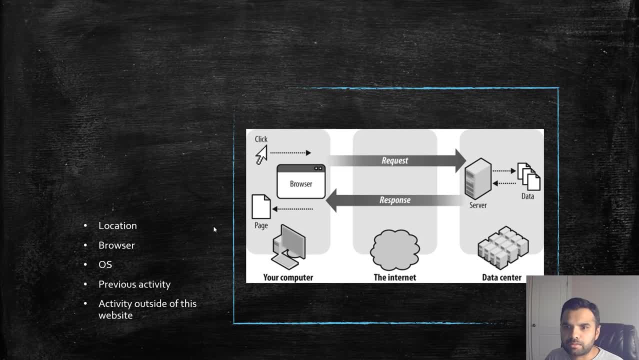 and os. that's like basic thing. any, any system, any, any website can track you down, so your, your privacy and anonymous anonymity is is going into the trash right away now. other thing which also uh systems like google and facebook can also track, is what are the previous activities that you have been? 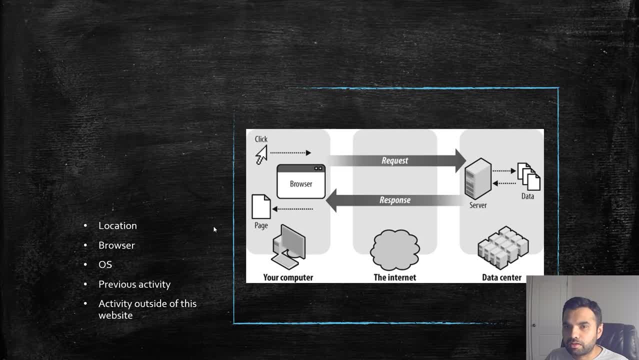 doing now. they can map, uh, what are the activities that you have done right now? and, based on your identity, it can also map what are the previous activities that you've done and and based on that, it can give you the advertisement that that's their main business. so 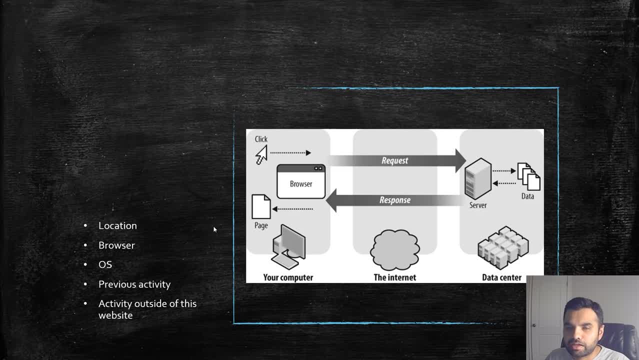 of course, they'll serve the advertised based on your liking and and your browsing history. uh, which is, which is fine. but then another thing is: activities outside of this website can also be tracked. so, for example, let's say, you do not have facebook profile or you do not have linkedin. 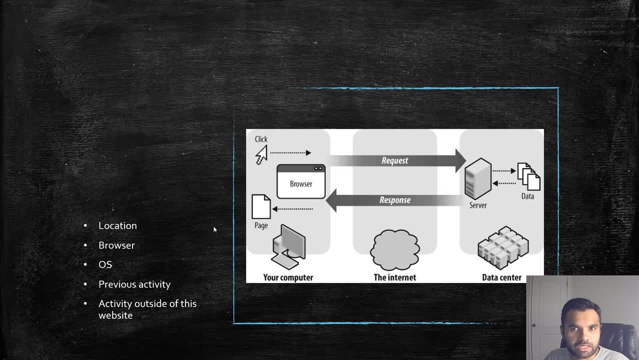 profile. but let's say you are visiting a website where it says, okay, share via facebook, linkedin or twitter or whatever. those website has a piece of code from this, this google, google co, this piece which is also tracking your activity. so, in the background, they are still going to make a profile. 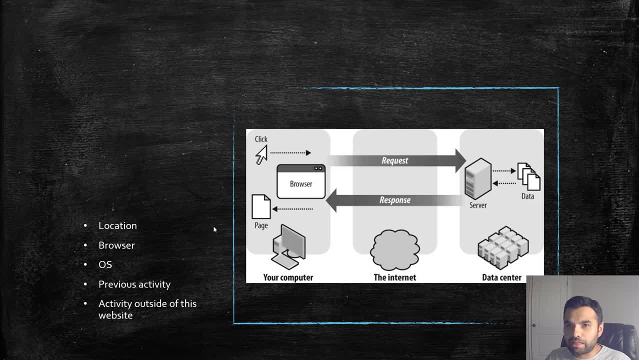 even though you do not have a public profile of facebook, and they will map the identity to you, uh, based on your activity. so it's not that only if you have the profile with the facebook or twitter, uh, they have your data. but no, irrespective if you are visiting any of the website where it's. 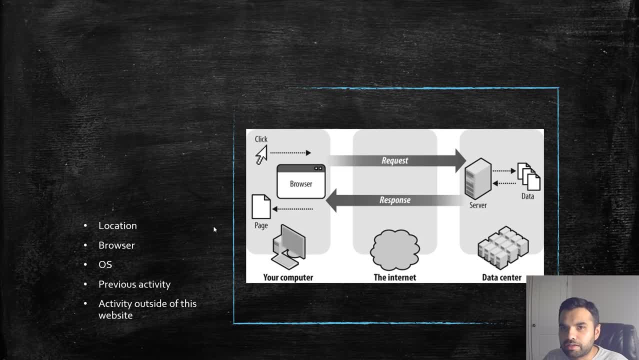 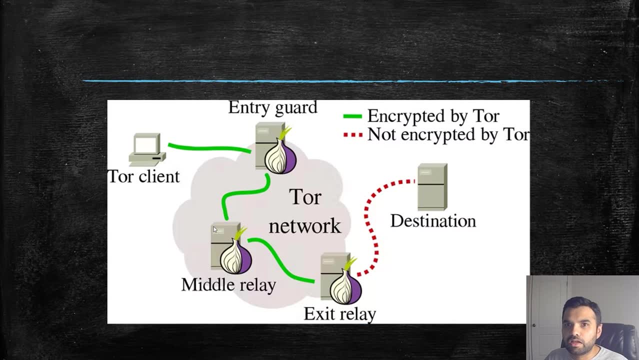 running the google or twitter code, your, your profile is still created and your activities are still being tracked. so that's why we need to use something like a tor, which is, uh, totally, uh, like you know, anonymous. so how, uh, tor pretty much works is like you have a tor client which is in your system, you have a tor browser. then tor has mainly. 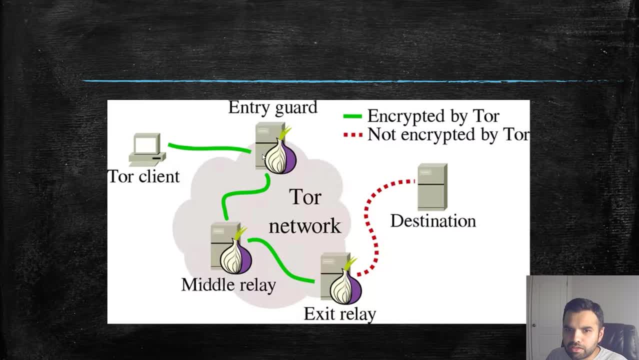 three intermediate server uh for any communication. so first uh the browser will will connect to the tor uh network and then it will connect to the another bounce off from that to the middle relay and then it will go to the exit and which will say uh request to the destination. now you must be wondering what are the green arrows and the red? 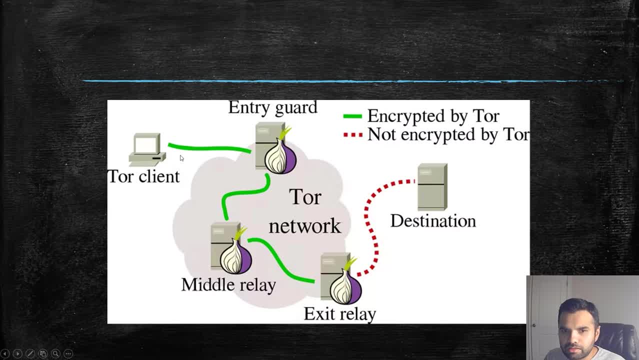 arrows, so the green arrows, so here this one. so, although it says encrypted over tor, but this one, uh, for example, tor client, you can have, like you know, https extension in your browser. uh, the site itself is uh tls protected, uh, anyway, so that's obviously encrypted. so tor will uh make sure. uh, so, even, like you know, let's say, your isp. 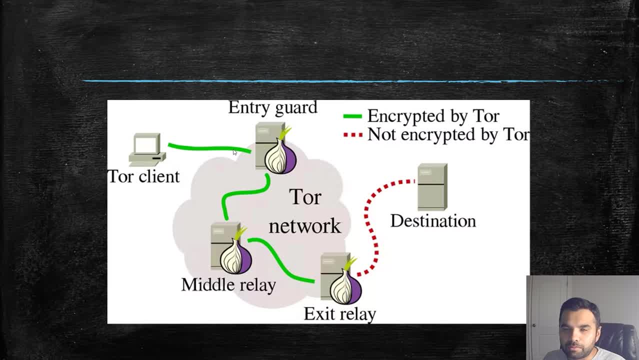 still tracks or perform a in the middle attack, uh, to intercept where the traffic is coming from or what you're trying to access? uh, they will only be able to see that you are trying to access the tor service. they won't know which end website that you are trying to access, such as googlecom. 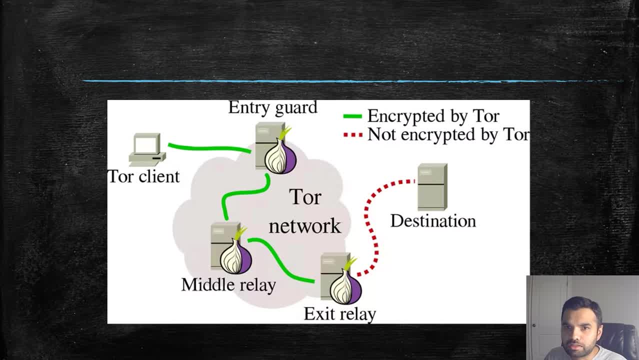 so that's one thing you definitely want to understand. so, even though, uh, you type googlecom, it will only see that you are accessing tor, and then it will go through three different servers. they have bunch of like in this network. they have tons of other servers, but for this 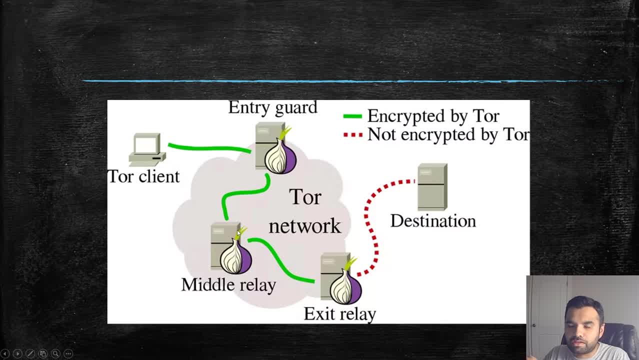 example: uh, for any request it's going to go through the three different servers and finally, when it reaches to the exit relay, uh, that's why the traffic is unencrypted. but that really doesn't matter, because at that time you are completely anonymous, because destination will only see. 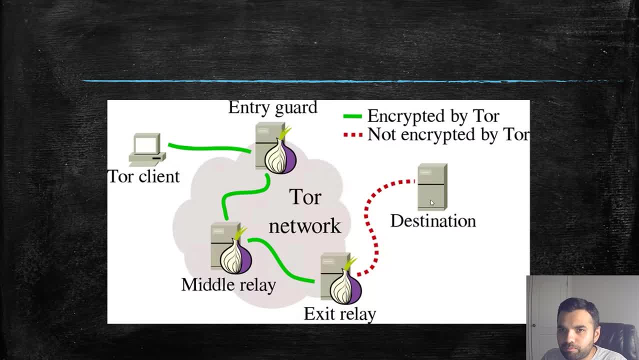 the last node, where the traffic or the request is coming in. it's not going to see where the actual- uh, like you know, it's not going to see where the client who actually made a request. that's why it's very anonymous in terms of how the traffic is reached to the destination and how the response is also received by the client. 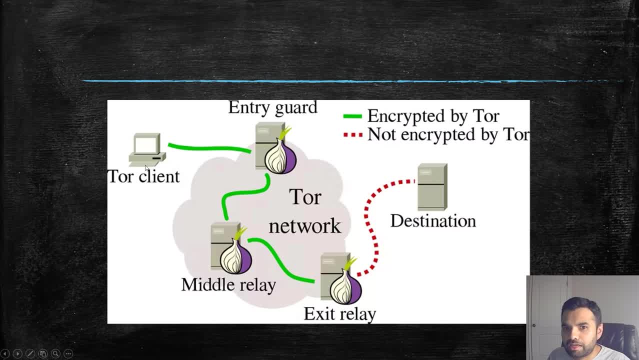 so that way again, like you know, when the response is received to the client, isp would not know which website or has sent the response back to the client. it's only going to see the tall record that it's going, like you know, sending a response back to the client. so this is, like you know, the 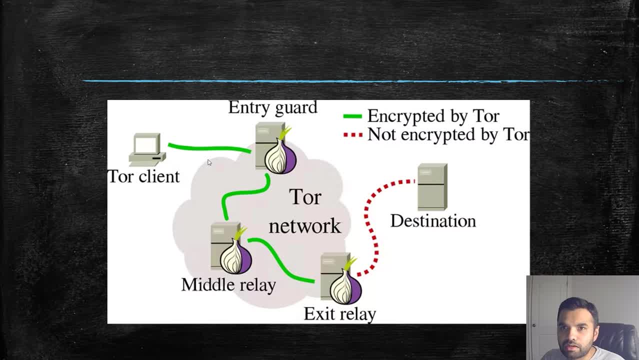 the main. uh, if you haven't, if you haven't tried tor yet, i would definitely highly recommend to do that. just download it. it's open source and you can play around and see, even even though if you are not interested in dark web or any services, but if you still want to keep your privacy and anonymity, 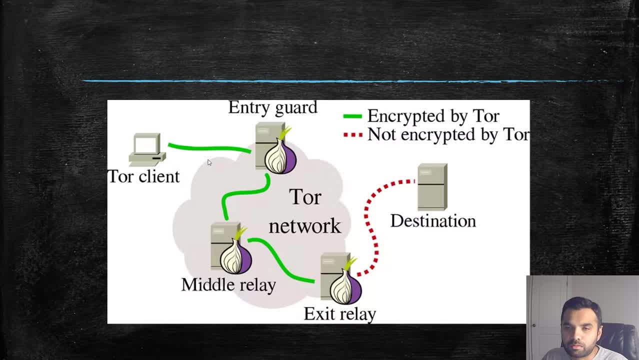 then, yeah, definitely go and and search for the tor browser and download and install it. it will provide you much more privacy than all the other browsers. but, yeah, that's all i wanted to talk about in this episode. i wanted to keep it very brief and in the future episodes i'll talk in more details on how the 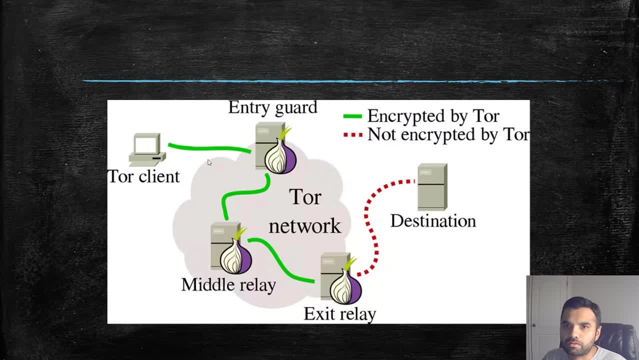 online routing works, and what are the services and how to access them, how to keep yourself secure, etc. etc. in this whole series. i'll create a new playlist for that so you can easily follow along. if you have any other questions, feel free to let me know. please hit the thumbs up button. 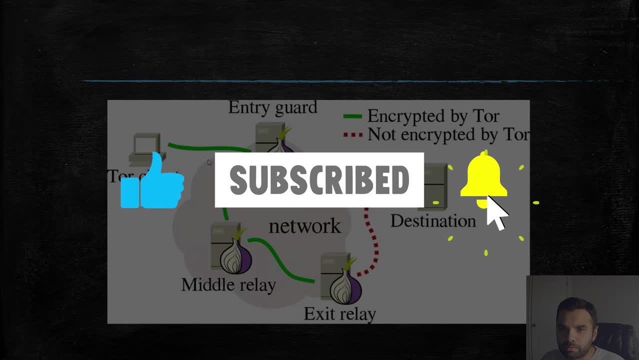 if you haven't already, subscribe to my channel and i'll see you all next monday. bye. 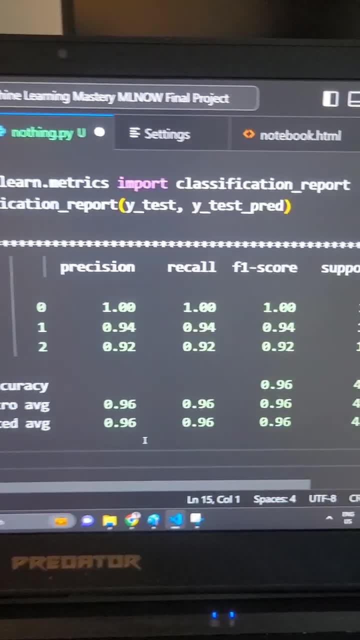 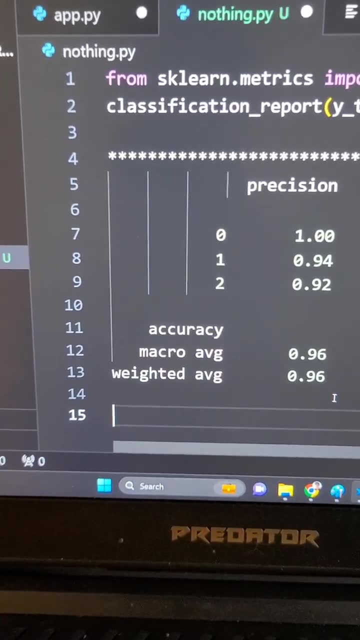 If you've used Scikit-learn, make sure you check this out. Scikit-learn's classification report is going to give you an entire analysis of all the important metrics of your machine learning model. So for each output- class 0,, 1, and 2, we're going to calculate the precision, the recall, the F1. 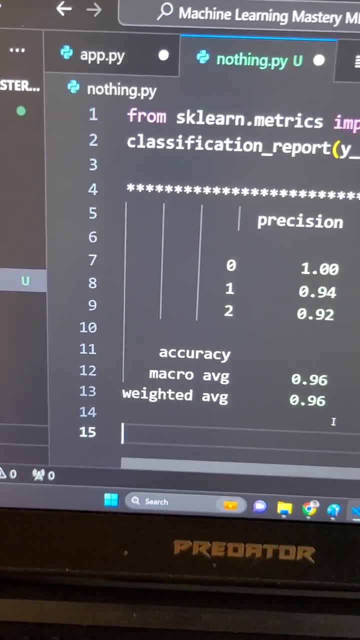 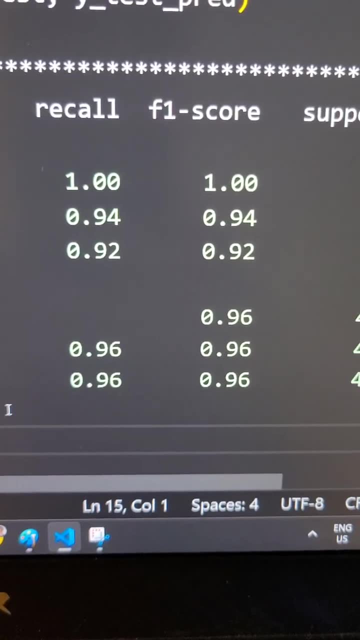 score and the support, which is just the number of examples. The only thing you really need to know about these numbers is that the closer they are to 1,, that means the model is doing better, and the closer it is to 0,, that means it's doing worse. Follow me for more, and if you don't, then